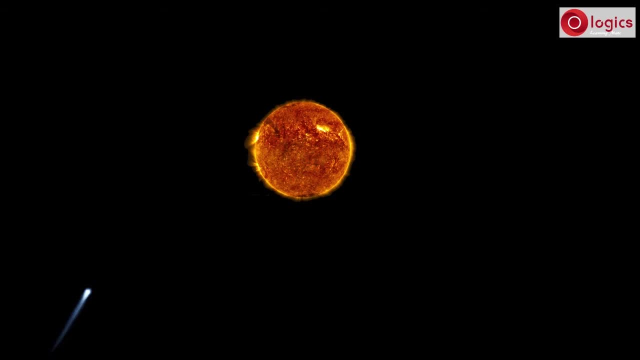 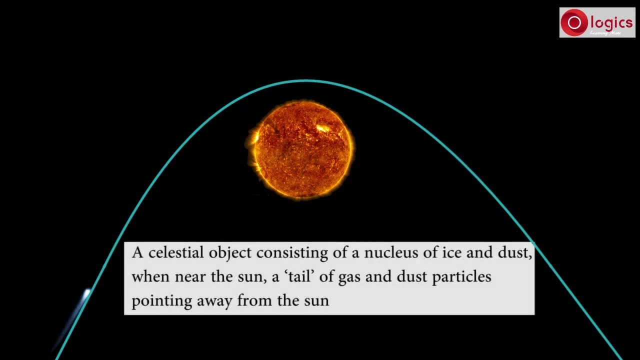 First and nucleus last. Comets revolve round the sun in highly eccentric orbit And have their origins from outer solar system. We can say comet is a celestial object consisting of a nucleus of ice and dust. When near the sun, a tail of gas and dust particles pointing away from the sun. 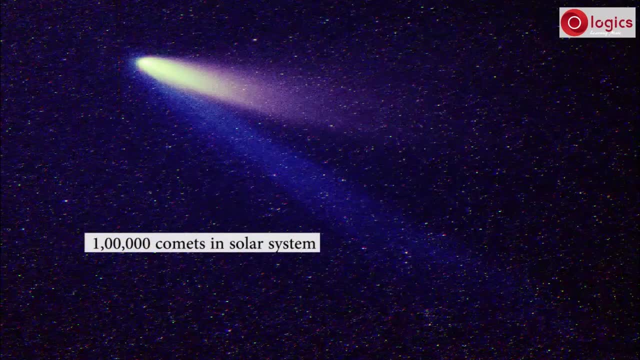 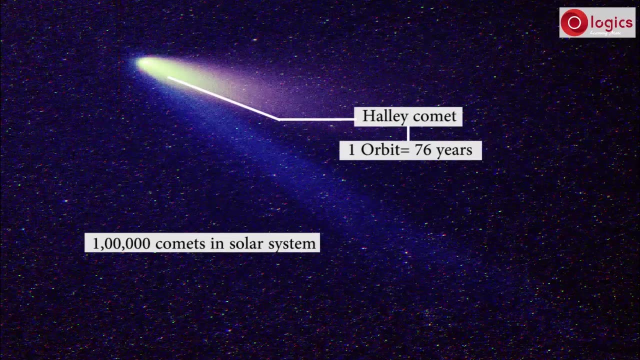 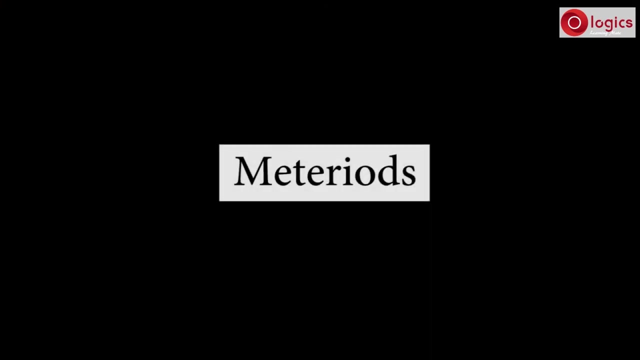 There are about 1 lakh comets in our solar system. Halley's comet is the most important one. It completes its orbit around the sun in 76 years, Last seen in the year 1986.. Let's understand about meteoroids. 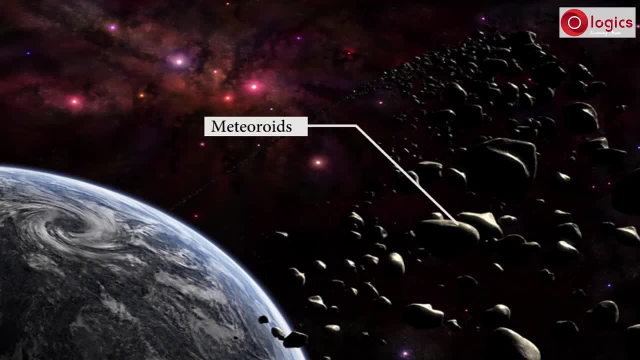 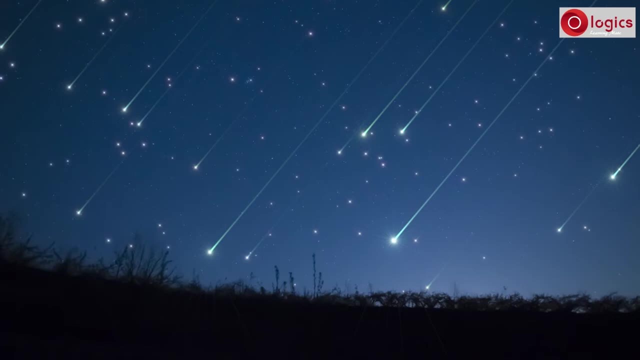 Meteoroids are the minute objects orbiting the earth. They are pieces of comets or asteroids which have collided. When meteoroids enter earth's atmosphere, they are heated up and burns Then a bright streak of light that flashes for a moment across the sky, known as meteors or shooting stars. 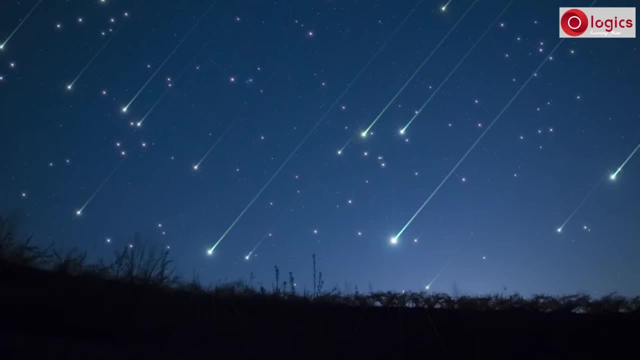 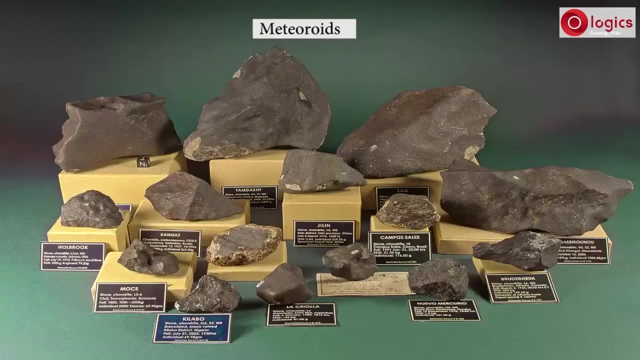 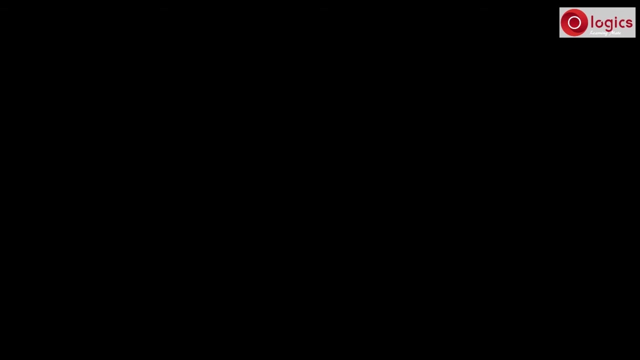 Some meteoroids are called meteoroids. Some meteoroids are called meteoroids. Many meteoroids survive in their journey through earth's atmosphere and fall on the earth's surface, creating craters. They are called meteorites. Let's understand about constellations. 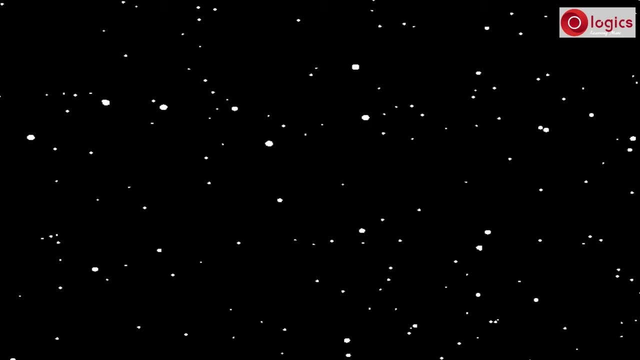 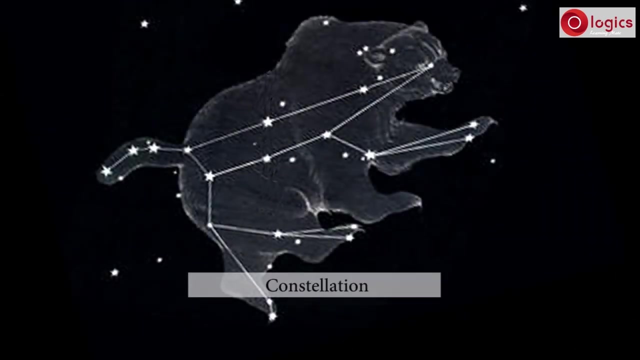 Observe It is a group of stars. These stars appears to be arranged in some pattern. Observe It is a group of stars in some patterns resembling some recognizable figure, In this case a bear. This group of stars is called a constellation. 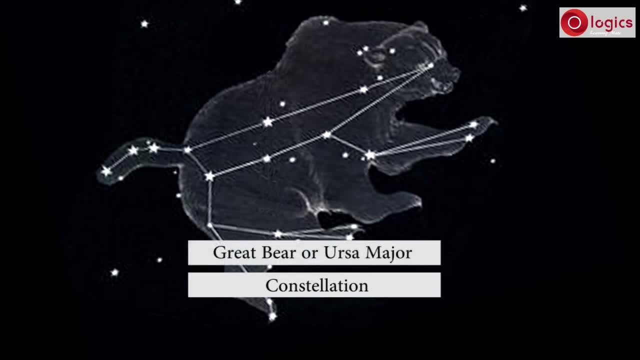 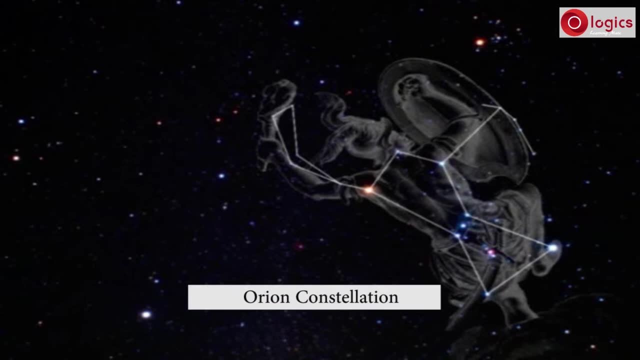 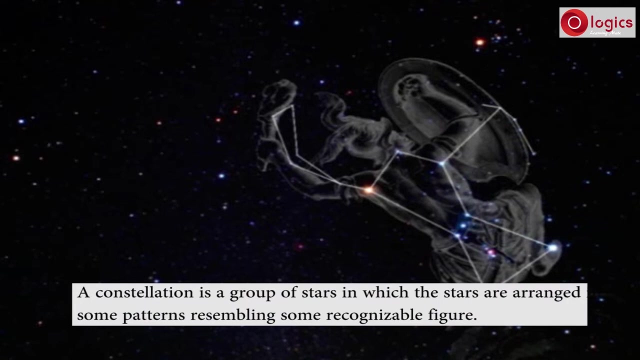 Here. this constellation is called Great Bear or Ursa Major. Similarly, another group of stars in different part of sky are named has different constellations. About 88 constellations are known so far. A constellation is a group of stars in which the stars are arranged in some patterns resembling 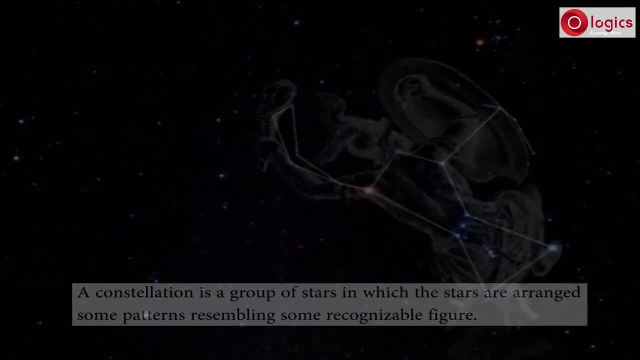 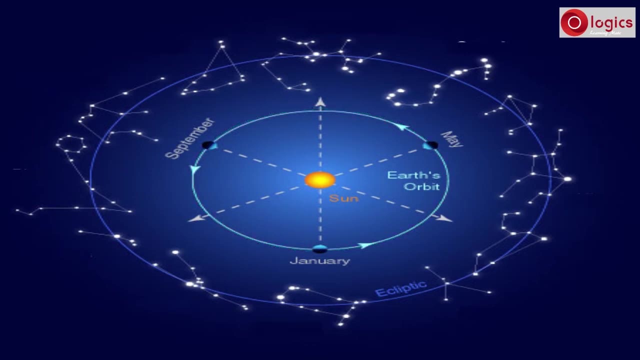 some recognizable figure Around Earth orbit. 12 constellations are named. They are: Aries, Taurus, Gemini, Cancer, Leo, Virgo, Libra, Scorpio, Saturn, Jupiter, Saturn, Aquarius, Sagittarius, Capricorn, Aquarius and Pisces. 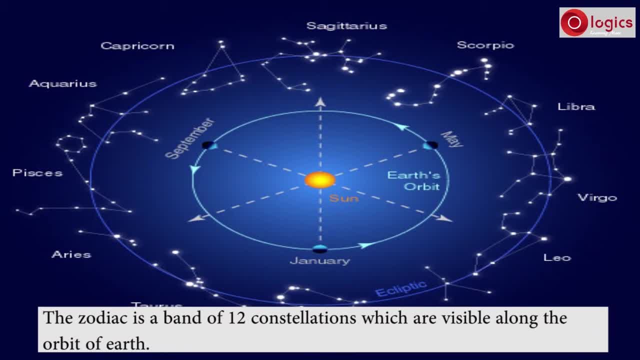 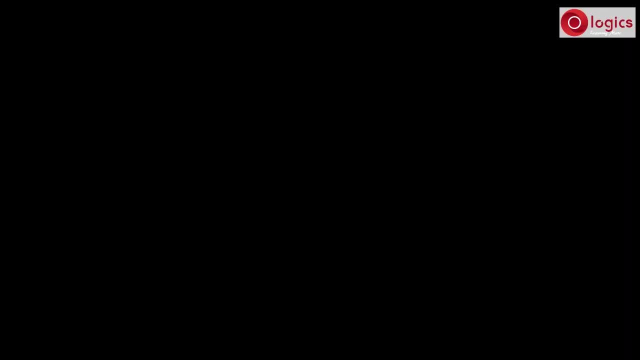 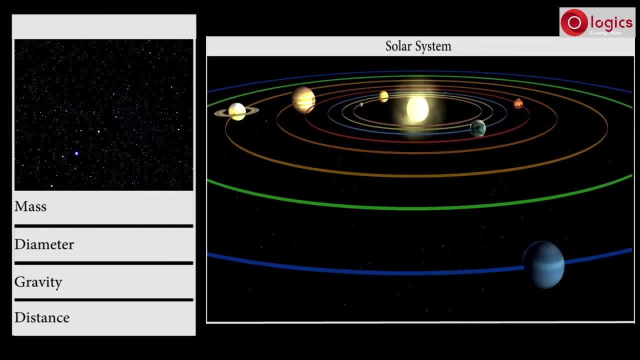 This band of 12 constellations called Zodiac. Lets know about planets in solar system in detail. The first planet in solar system is Venus. The second planet in solar system is Mercury. Mass of Mercury is 3.285 into 10 to the power, 23 kilograms. 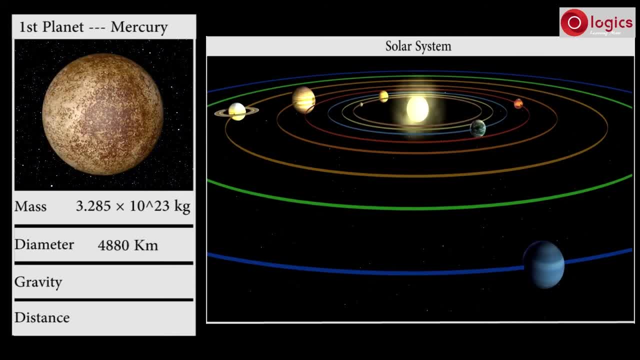 Its diameter is 4880 kilometers, Gravity on Mercury is 3.7 meter per second square And distance of Mercury from Sun is 57.91 million kilometers. The second planet in solar system is Venus. Its mass is 4.867 into 10 to the power, 24 kilograms. 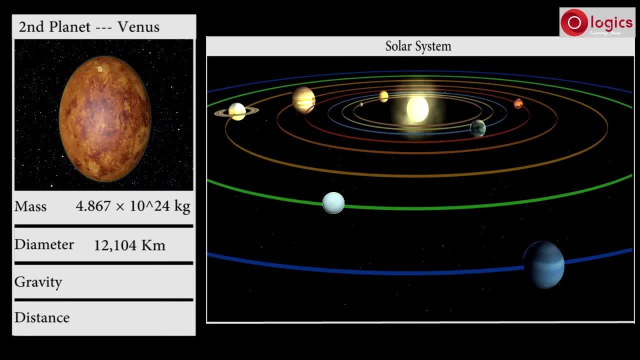 Its diameter is 12104 kilometers. Gravity on Venus is 8.87 meter per second. square 4.867 into 10 to the power 24 kilograms. Its diameter is 12104 kilometers And 8.2 million kilometers distance from sun. 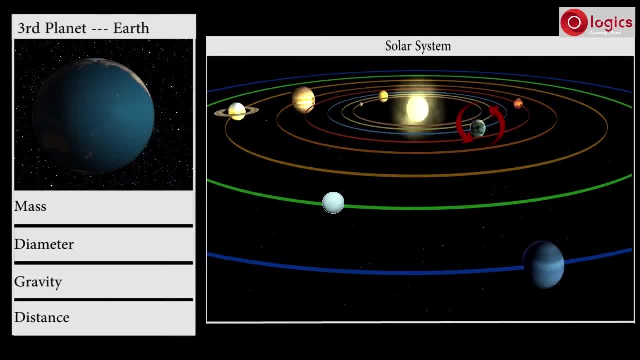 The third planet in our solar system is our own planet, earth. Its mass is 5.972 into 10 to the power, 24 kilograms. Earth's diameter is 12,742 kilometers. Gravity on earth is 9.807 meter per second square. 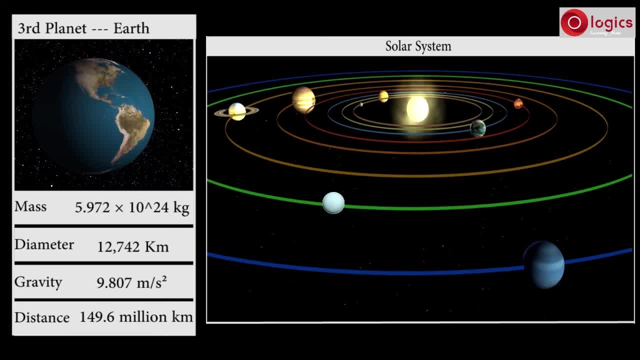 And earth is 149.6 million kilometers away from sun. Fifth planet in solar system is Mars. Its mass is 6.39 into 10 to the power 23 kilograms. Mars diameter is 6,780 kilometers. Gravity on Mars is 3.711 meter per second square. 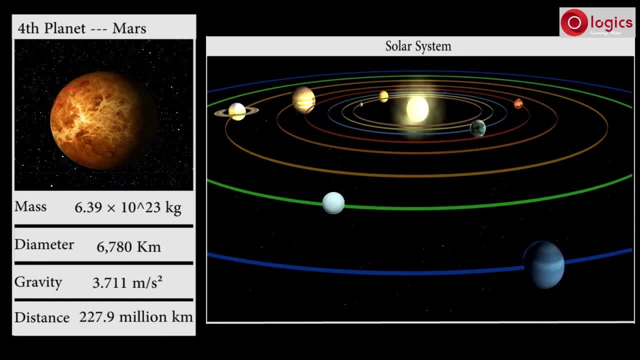 And Mars is 227.9 million kilometers away from sun. The sixth planet in our solar system is Jupiter. Its mass is 6.7 into 10 to the power: 24 kilograms. Its mass is 1.898 into 10 to the power: 237 kilograms. 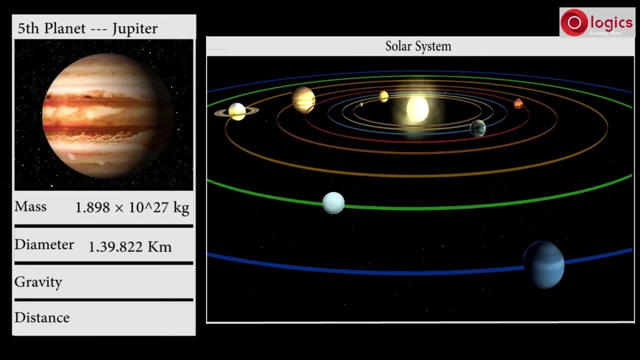 Its diameter is 139822 kilometers. Gravity on Jupiter is 24.79 meter per second square. Jupiter is 728.5 million kilometers distance as distance from Sun. The sixth planet in our solar system is Saturn. Its mass is 5.683 into 10 to the power, 26 kilograms. 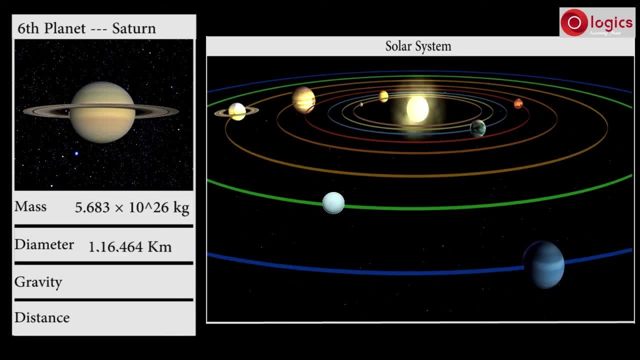 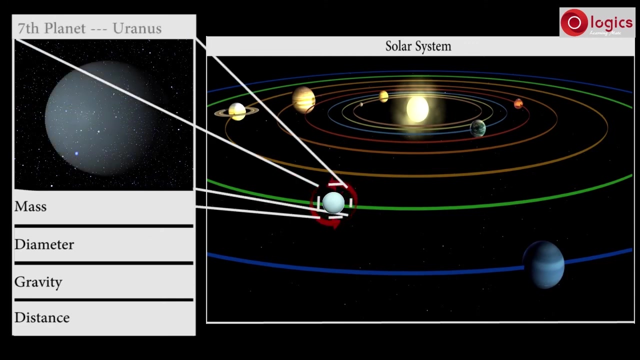 Saturn's diameter is 116,464 kilometers. Gravity on Saturn is 10.44 meter per second square And Saturn is 1.429 billion kilometers from Sun. The seventh planet in our solar system is Uranus. Its mass is 8.681 into 10 to the power 25 kilograms. 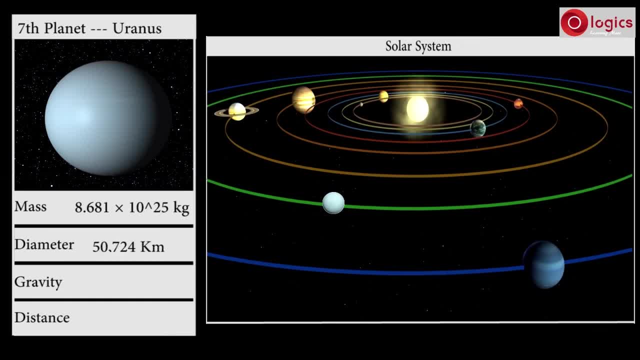 Uranus's diameter is 8.681 into 10 to the power 25 kilograms. Uranus's diameter is 8.681 into 10 to the power 25 kilograms. Its mass is 50,724 kilometers. Gravity on Uranus is 8.69 meter per second square. 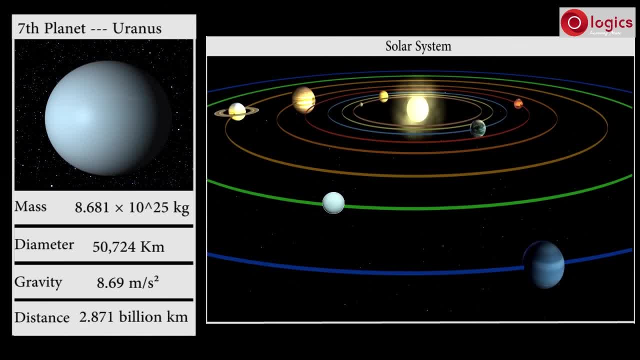 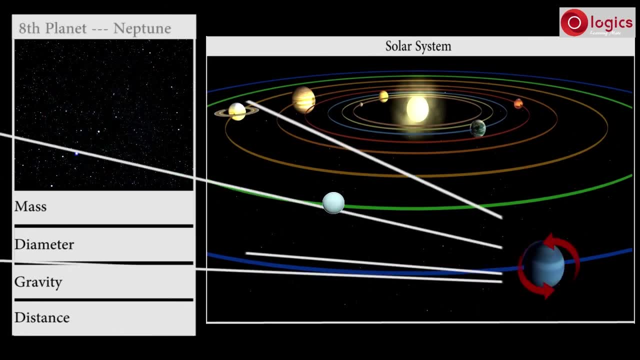 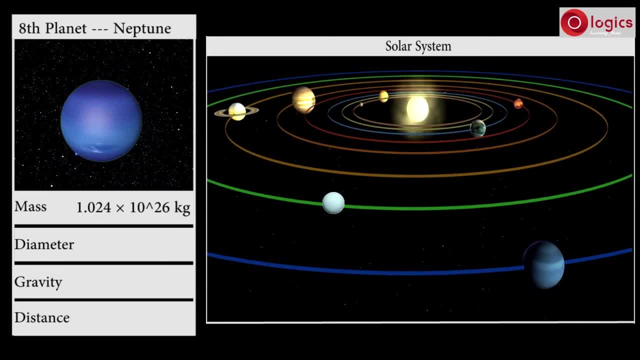 Its mass is 1.024 into 10 to the power, 26 kilograms. Neptune's diameter is 49,244 kilometers, Gravity on Neptune is 11.15 meter per second square And distance of Neptune from Sun is 4.498 billion kilometers. you. 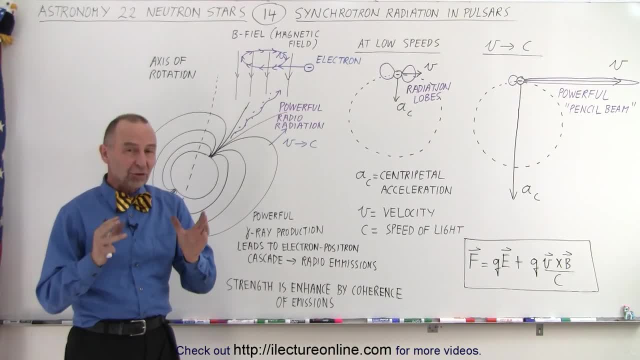 Welcome to iLectra Online. When we actually try to explain how those radio beams are produced in pulsars, well, it's not as easy as it may sound. You hear terms such as synchrotron radiation, and how does it actually work? Well, let me try to explain a few fundamentals in order to make 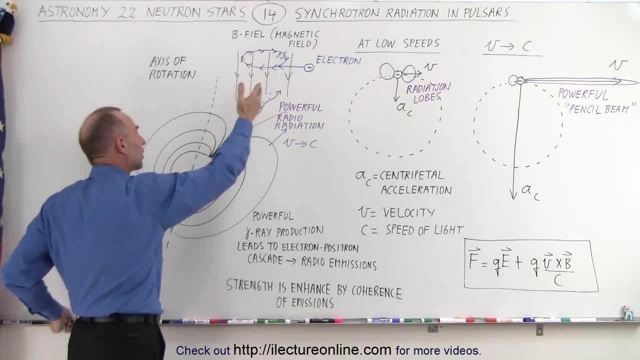 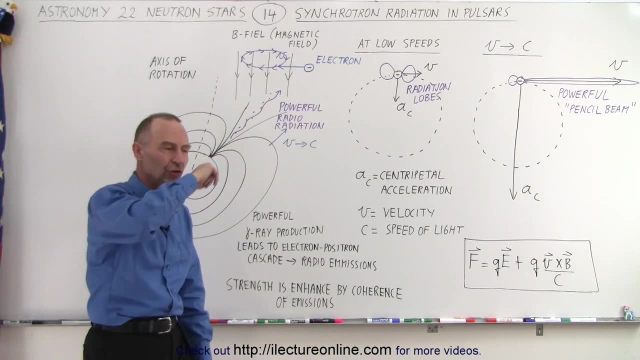 it easier to figure out how radio beams are sent in both directions along the axis of the magnetic field. So, first of all, synchrotron radiation is produced when charges move around in circles. Now, when you have something that looks like this, where, let's say, an electron goes around in circles, 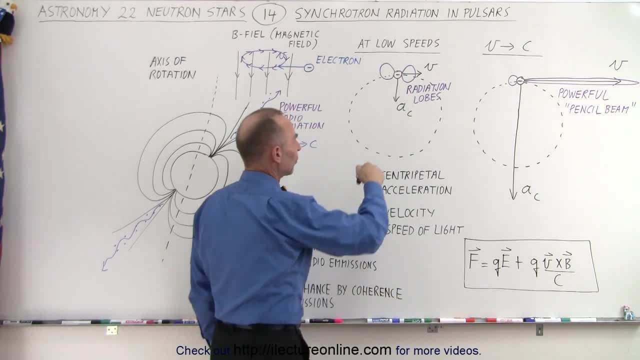 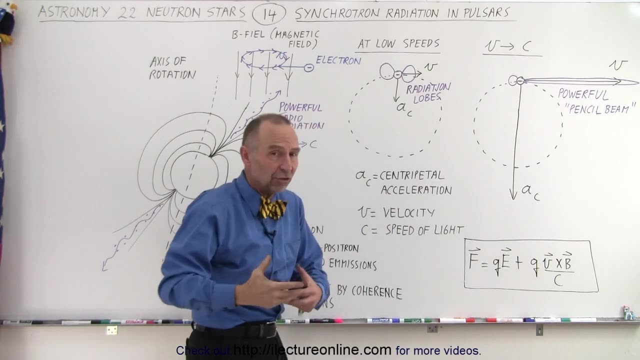 we have what we call centripetal acceleration, That's acceleration towards the center of the rotational motion, which causes radio radiation or not necessarily radio radiation. it depends upon the speeds and the frequency. We have radiation going in both directions and the 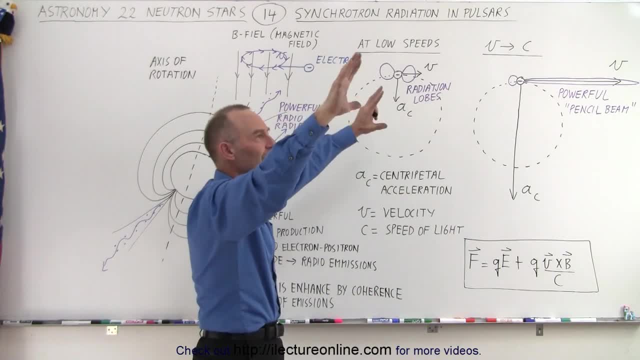 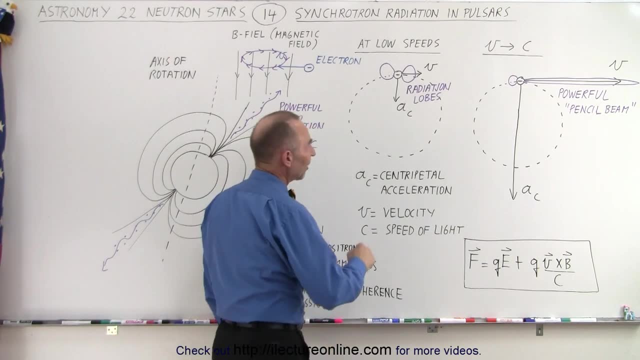 direction is not very precise. In other words, radiation is being sent in all directions, in one to one direction, and in all directions, all angles, I should say in the other direction. But as the object begins to move faster and the speeds of the object, like electrons, start approaching the speed of light, 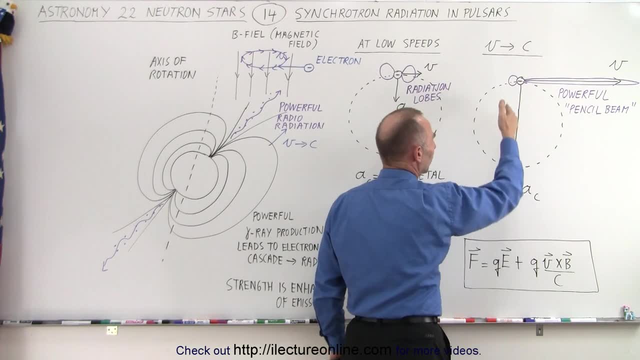 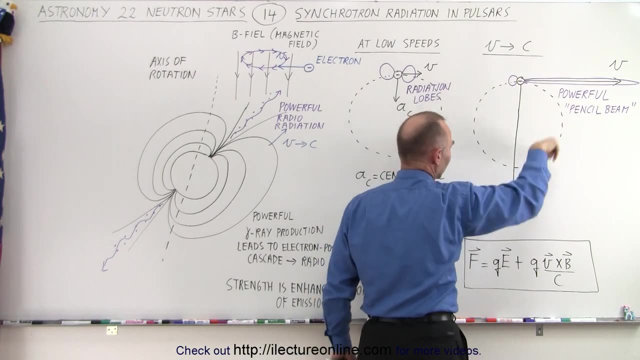 then we have a much greater what we call centripetal acceleration and we have in the direction of travel, and of course you can see that this pencil beam is going to go around like that, as it goes around, but in the direction of motion of the charge. 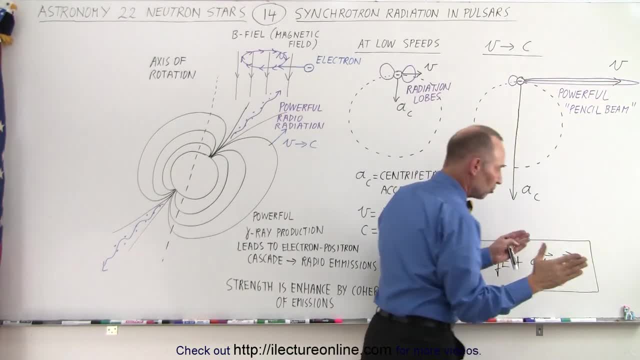 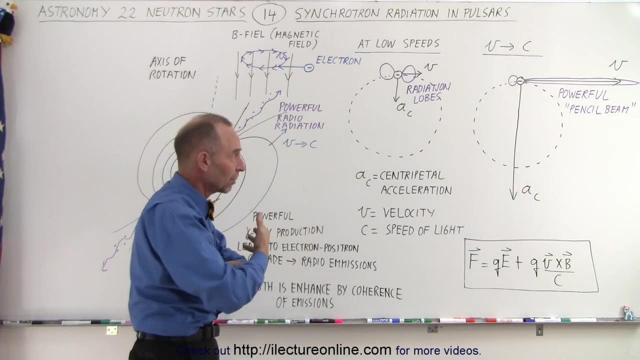 we have a much more powerful and much more directed and much more narrow beam of radiation that is emitted from the charge- And of course we're not talking about one charge, but we're talking about gazillions of charges. moving that direction. We have a pencil beam of radiation.